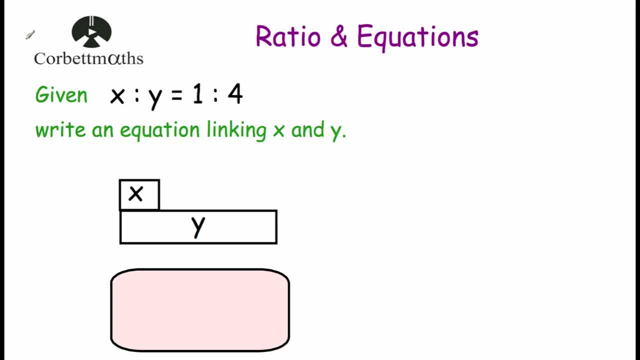 Hi, welcome to this CodeMaths video on ratio. In this video, we're going to look at how to write a ratio as an equation and how to write an equation as a ratio. Now, given the context of the question, you might be asked to write a ratio as a formula or a linear function, but the technique is the same as how to write a ratio as an equation. 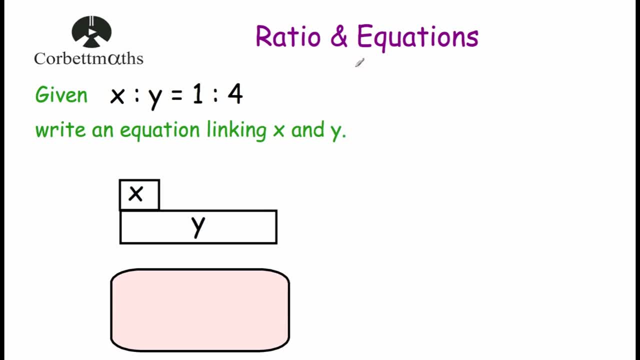 So that's what I'm going to talk about in this video. I'm going to talk about how to write ratios as equations. Now, there's an example later where we write a ratio as a formula, but it's the same approach. Okay, let's have a look at our first question. 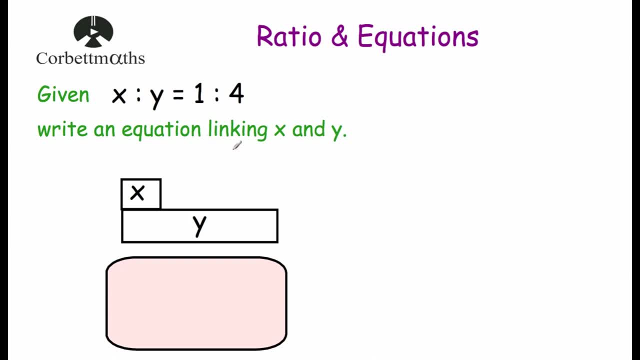 Given the ratio of x to y is 1 to 4, write an equation linking x and y. So x and y represent two numbers and we know that whenever we write them as a ratio and simplify it, we get that the ratio is 1 to 4.. 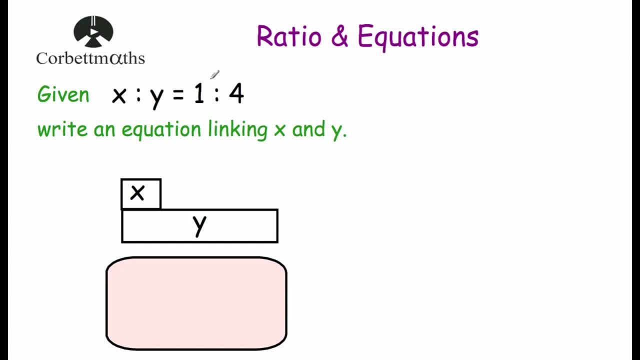 In other words, the value for y is 4 times larger than the value for x. So x could be, for instance, a number like 100, y could be 400, and if you simplified that ratio, you would get 1 to 4.. 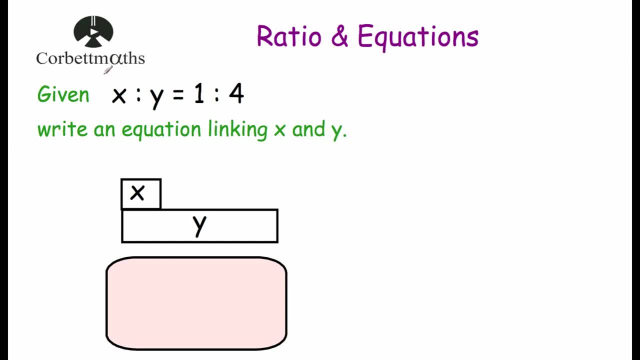 Or x could be equal to 5 and y is equal to 20, or x could be equal to 2 and y is equal to 8.. As long as it cancels down to 1 to 4,, they could be your values for x and y. 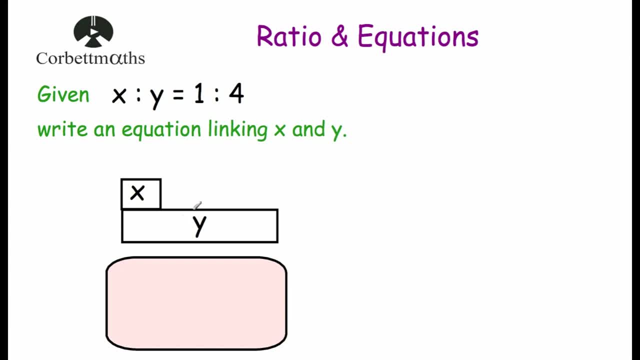 Now we need to write an equation linking x and y. So we know the value for y is 4 times larger than the value for x. So if we multiply the value of x by 4, we will find that that's the same as the value for y. 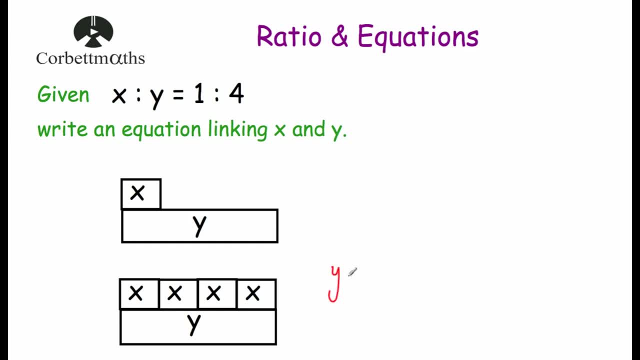 So that will give us an equation We will have the value for y. y is equal to 4 times the value of x, And that's it. So our equation would be y equals 4x. But what's useful to notice there is there's a little bit of a shortcut. 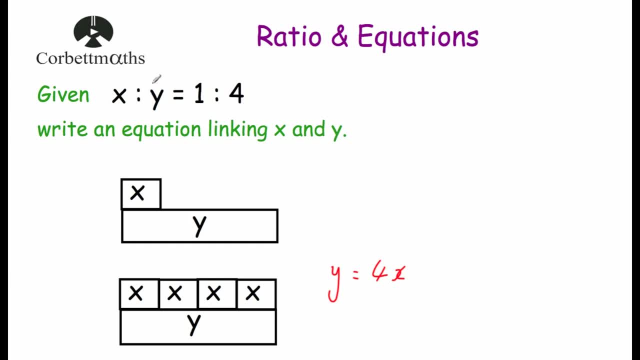 If we multiply the x by the y number in the ratio and we multiply the y by the x number in the ratio, that would give you an equation: y times 1 is y and x times 4 is 4x. so y equals 4x. 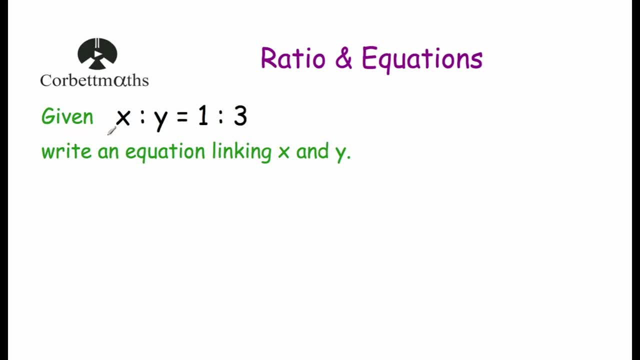 Okay, let's have a look at another example. So our next question says: given that the ratio of x to y is 1 to 3, write an equation linking x and y. So we've got two values, x and y, and we know that if we simplify that ratio we'll get 1 to 3.. 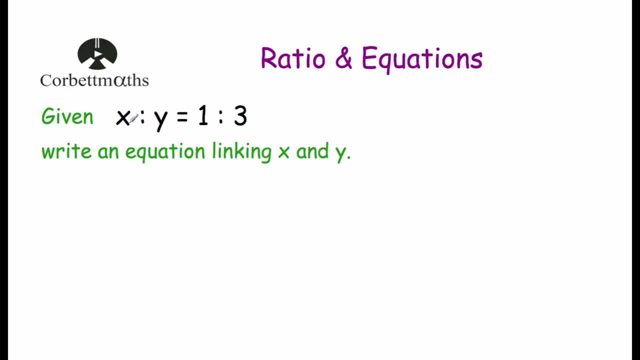 In other words, the y number is 3 times larger The x number. So it could be, for instance, 20 and 60.. So that means that if we multiply this x number by 3, we will get the y number. 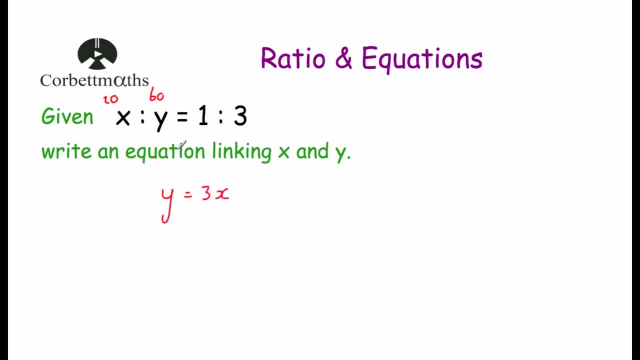 So we know that y equals 3 times x. Or we could use our shortcut that if we multiply x by the y number in the ratio 3, and the y by the x number in the ratio the 1,, we will get y equals 3x. 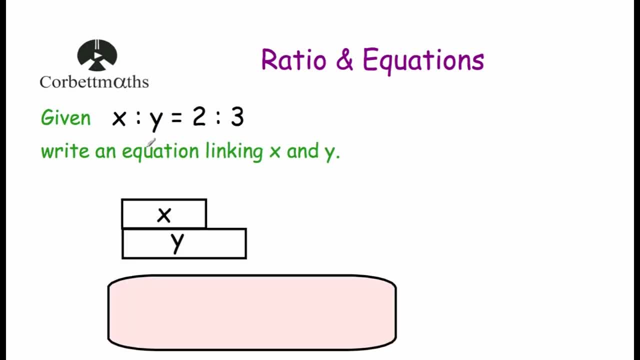 And that's it. So let's have a look at our next example. So our next example says: given the ratio of x to y is equal to 2 to 3, write an equation linking x and y. So x and y are two numbers that when we write them as a ratio and simplify it, we get 2 to 3.. 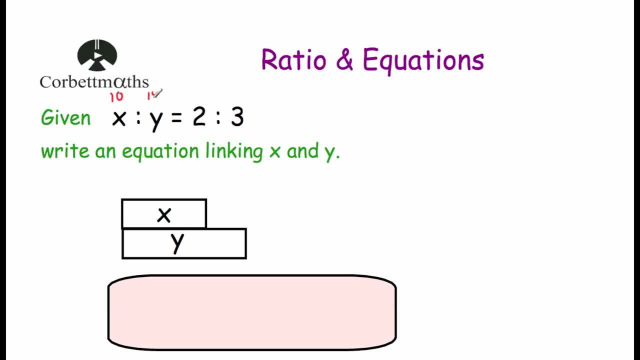 So that means, for instance, x could be equal to 10 and y could be equal to 15.. And if you divided both of those numbers by 5, you get 2 to 3. And they could be any numbers that would simplify down to be 2 to 3.. 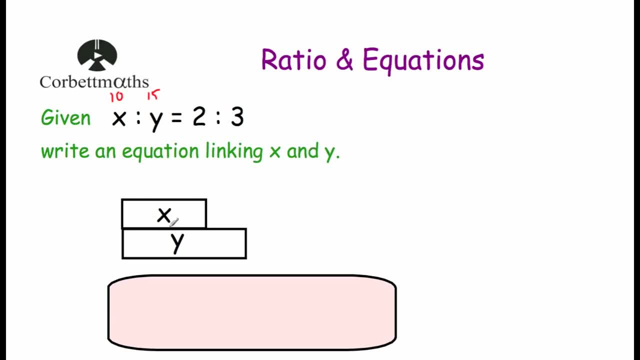 Now we want to find an equation linking them. Now we've got this value for x and the value for y, And if you multiplied the value for x by the y number in the ratio, the 3,, and if you multiplied the y value by 2,, 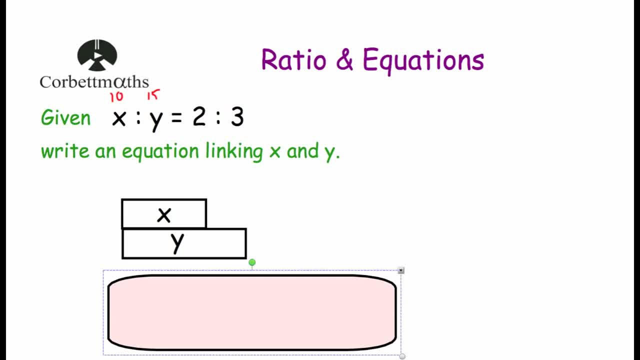 the x number in the ratio, you would find that they would be equal to each other. So, for instance, if x was equal to 10, you would get 30. And if y was equal to 15, you would get that's equal to 30 also. 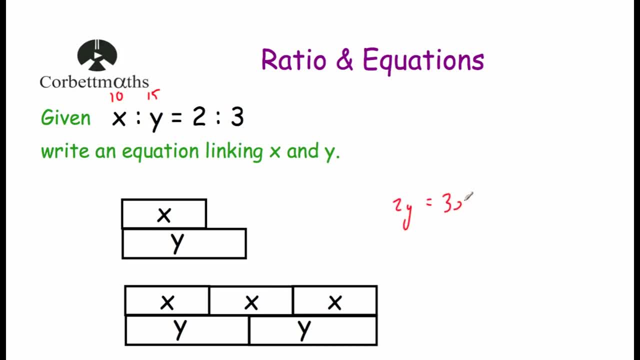 So that would be our equation: that 2y is equal to 3x. And again we could have taken our shortcut. We could have just multiplied the y by the x number in the ratio. So 2 times y is 2y. 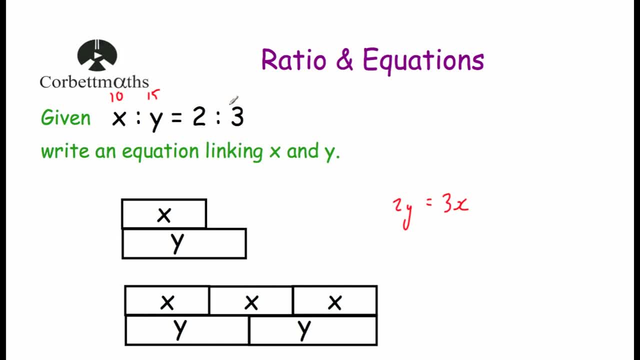 And we could take our x and multiply by the y value in the ratio, the 3, and then get that's equal to 3x. So 2y equals 3x. Now you might want to be able to make why the subject. 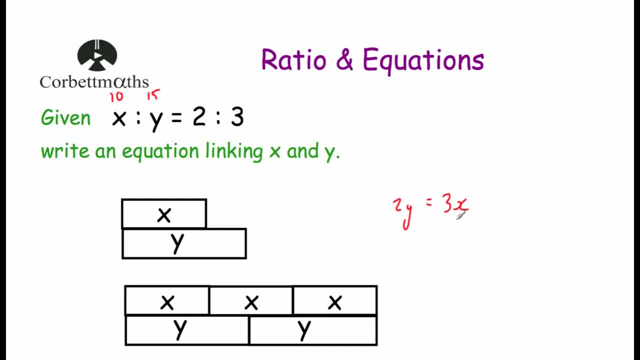 And if that was the case, you would just divide both sides of the equation by 2.. Or if you wanted to make x a subject, you could just divide both sides of the equation by 3. And that would help you make either one the subject. 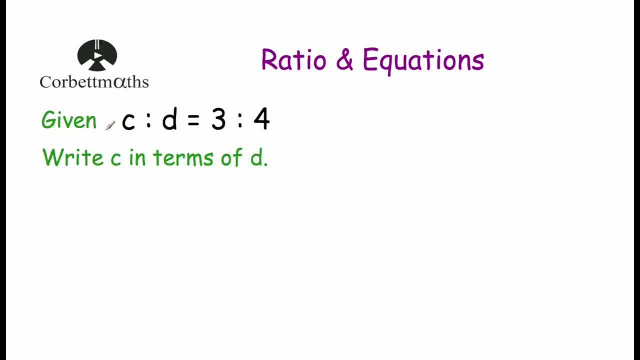 Okay, let's have a look at our next example. So our next question says: given that the ratio of c to d is equal to 3 to 4, write c in terms of d. So this time we're going to take our shortcut. 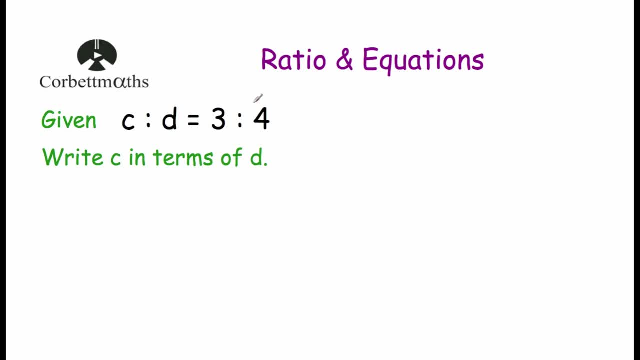 We're going to take our c and we're going to multiply it by the d number in the ratio, the 4. So that would be 4c, And we're going to then put our equal sign And then we're going to take our d. 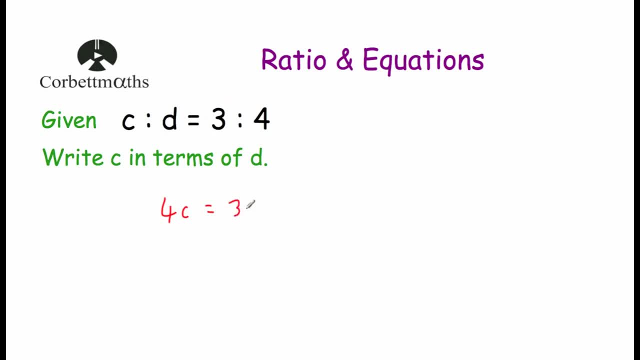 and times it by the c number in the ratio, the 3.. So that would be 3d. Now we've been asked in this question to write c in terms of d. So we've got our equation, or formula, depending on the context. 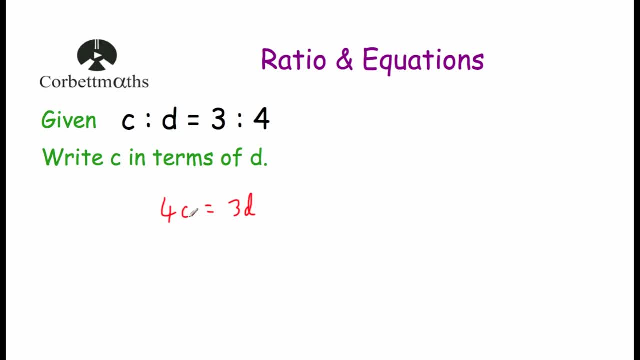 And we want to write c as a subject. So we want to have just c on its own here, So we don't want the 4.. So we're going to divide both sides by 4.. So divide by 4 and divide by 4.. 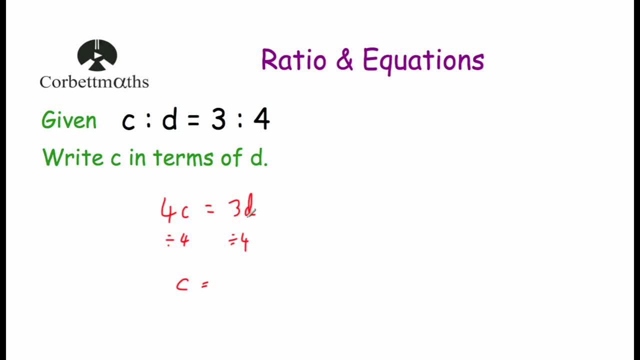 And that would give you that c equals. Now we could write 3d over 4.. So you could write this 3d over 4.. 4 like that, if you wanted to. I personally tend to just write: do the 3 divided by 4 to get 3 quarters. 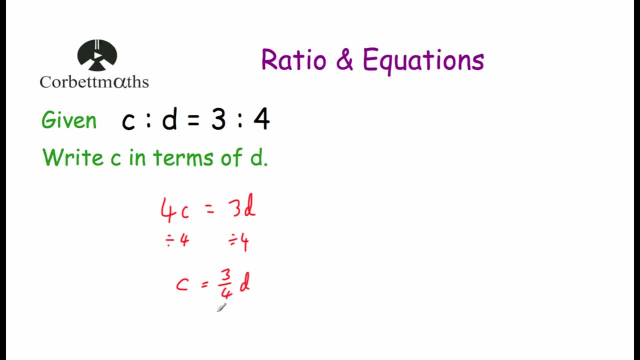 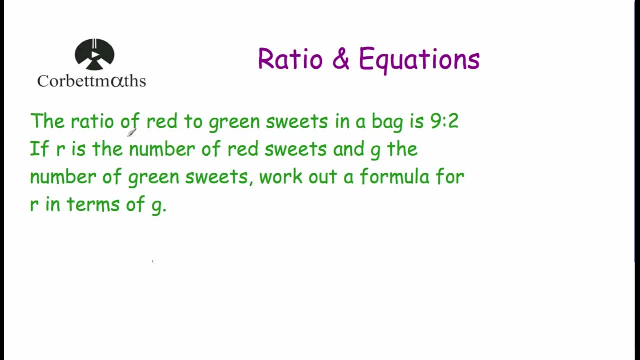 And then put d. So that just says that c is equal to 3 quarters of d, And that's it. So that's c in terms of d. Okay, let's have a look at our next question. Next question says the ratio of red to green sweets in a bag is 9 to 2.. 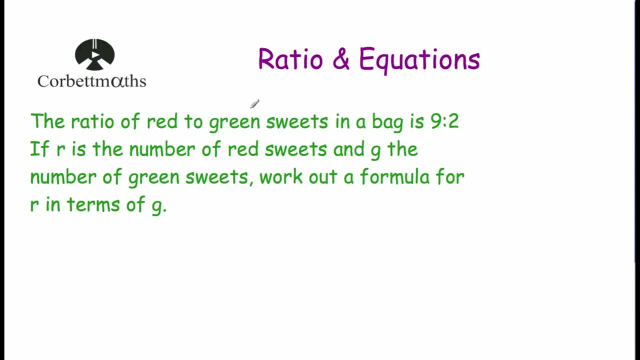 And if r is the number of red sweets and g is the number of green sweets, work out a formula for r in terms of g. This question mentions formula rather than equation, But remember, it's the same, It's the same approach. 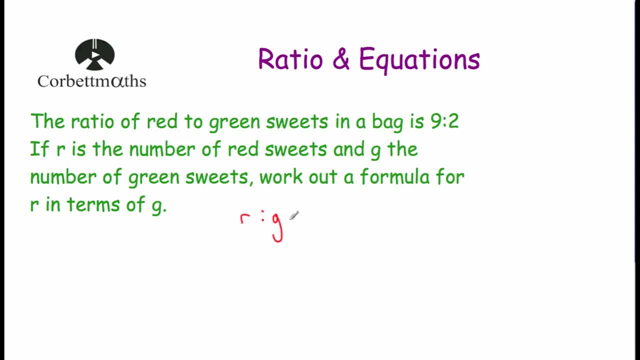 And we've got the. it's, the ratio of r to g is equal to 9 to 2.. And we want to write that as a formula. So what we're going to do is we're going to take our r and we're going to multiply it by the g number in the ratio, the 2.. 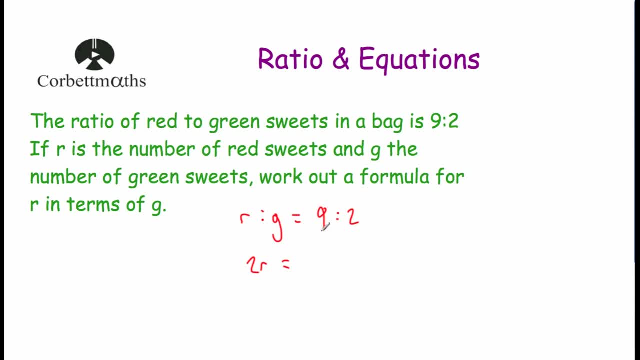 So that's 2r. And then we're going to take our g and multiply it by 9, the r number in the ratio. So we get 9g. Now we want our formula for r to be in terms of g. 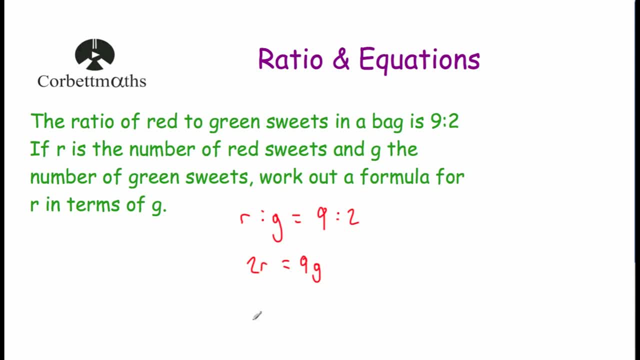 So we want r to be the subject. So we're going to divide by 2 and divide by 2.. So we're going to write: r equals 9 over 2.. Now we could have written: r equals 9g over 2.. 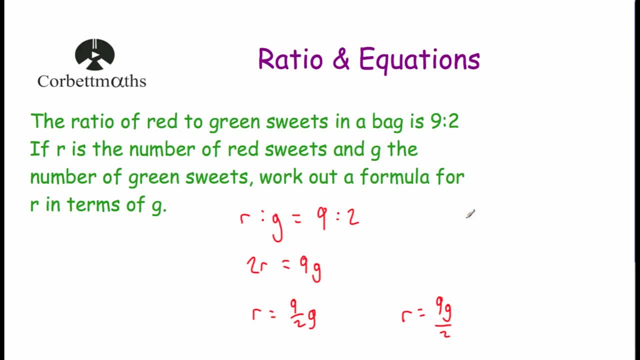 I tend to write the version on the left, but it's up to you. Okay, So we've looked at how to write a ratio as an equation. Let's see how to write an equation as a ratio. So here we've got an equation. 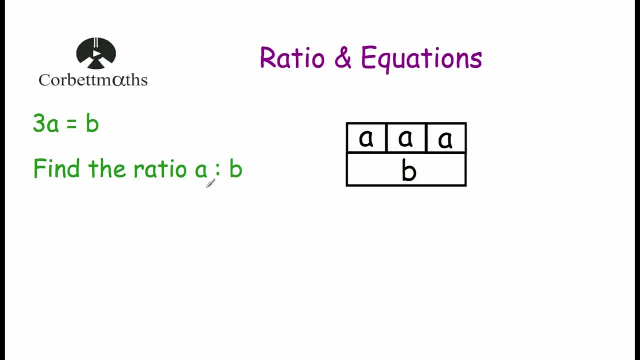 We've been given: 3a equals b And we've been asked to find the ratio of a to b. So this equation tells us that if we multiply a by 3, we get b. So in other words, b is 3 times larger than a. 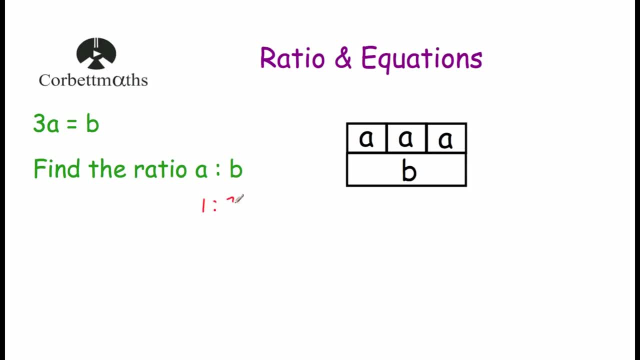 And if we want to write that as a ratio, we'll just write 1 to 3, b is 3 times larger than a And if we have a look at our equation, there is a shortcut again. If you've got 3a and b, remember b is just 1b. 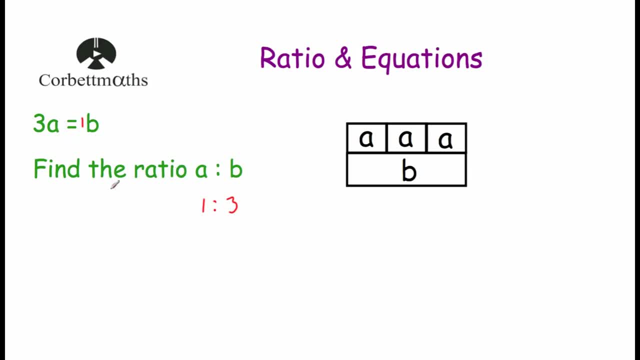 Then if we swap those numbers around, we can get our ratio really quickly. So we've got: our a is going to be 1, and our b in the ratio is going to be 3.. So 1 to 3.. Let's have a look at another question. 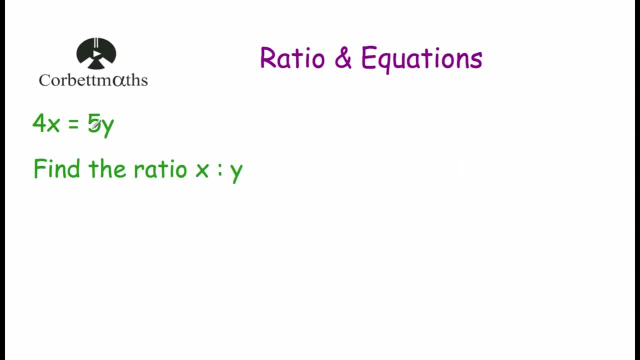 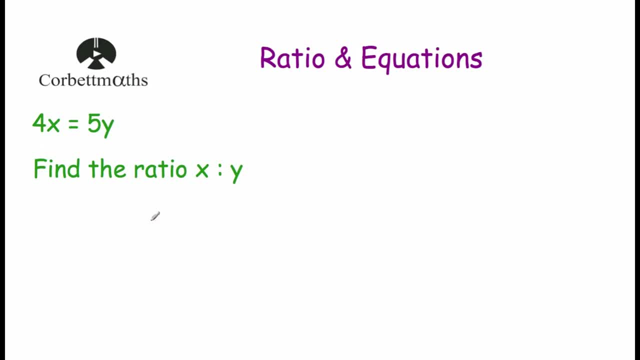 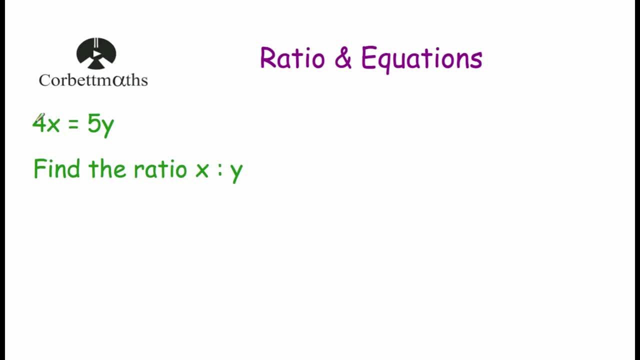 So we have got the coefficient of x. the number in front of the x is 4.. So that's going to be our y value in our ratio, And then the number in front of our y is 5.. So that'll become our x value in our ratio. 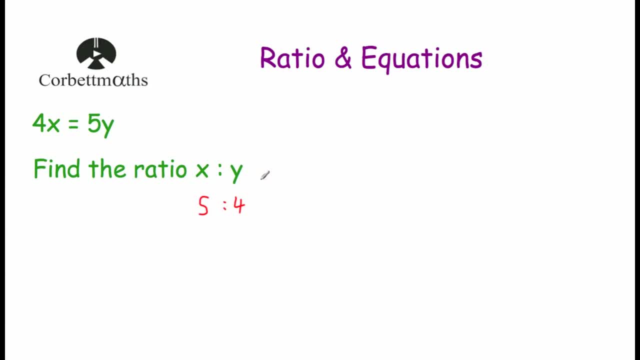 And that's it. So the ratio of x to y would be 5 to 4.. So let's have a look at our last question. So our last question says 6x plus 4y equals 7y minus x, And we've been asked to find the ratio of x to y. 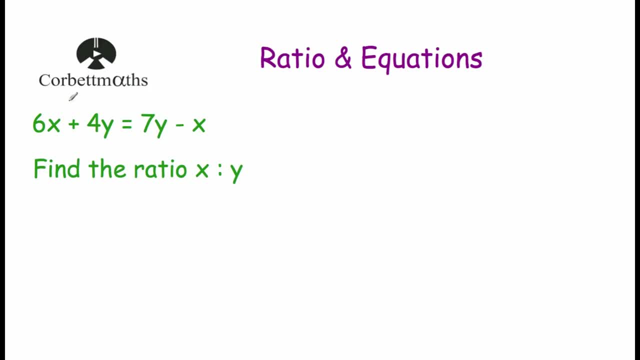 So what we're going to do here is we're going to get all bring all our x's to one side and all our y's to the other. so let's write down our equation: 6x plus 4y equals 7y minus x, and what we're going to do is we're going to 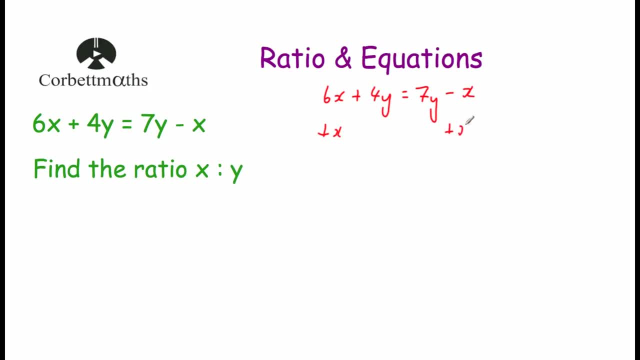 add x to both sides to begin with. so add x and add x, so we would get 7x plus 4y equals 7y. now we want to get rid of this plus 4y, so let's subtract 4y from both sides, so that would give us: 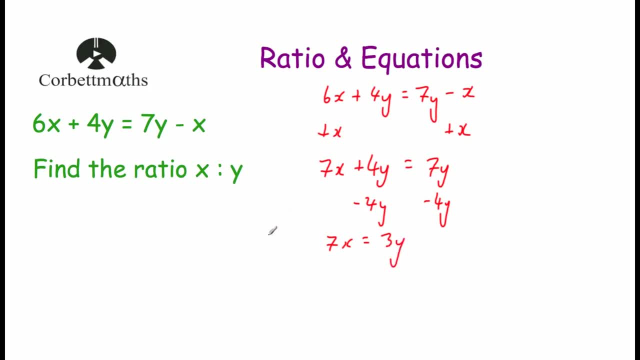 7x equals 3y. now we want to write this as a ratio of x to y. so what we're going to do is we're going to look at our numbers in front of our x and our y and we're going to swap them around. so, for our x, 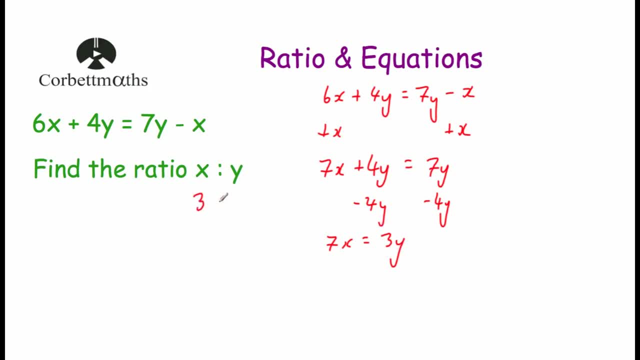 we will look at the number in front of our y, our coefficient of y, which is 3, and for our y, we will look at our coefficient of x, which is 7. so the ratio of x to y would be 3 to 7, and that's it. 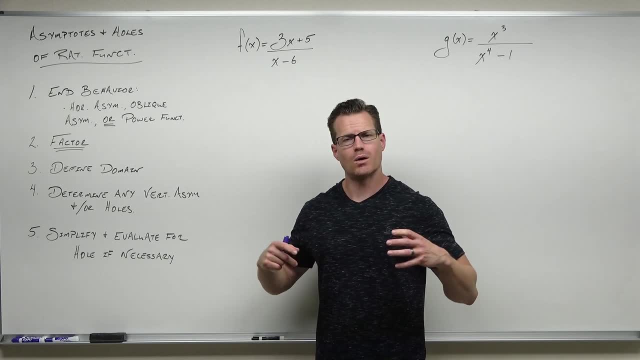 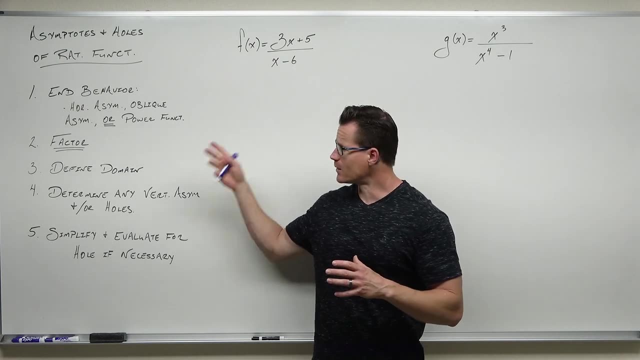 Hey there, welcome to another video. So this video is all about putting together the ideas that last like four or five videos. We are going to just basically be practicing. I'm going to give you an outline of structure on how to find all the asymptotes and holes in a function. We're going to